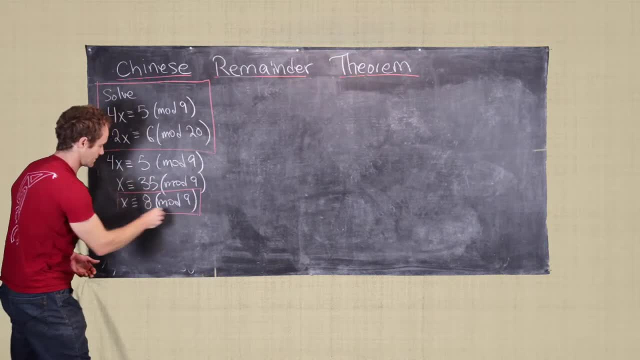 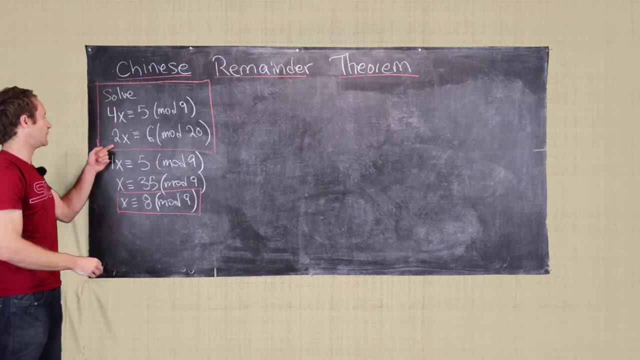 Good, We've simplified. 4x is congruent to 5 mod 9, down to x is congruent to 8 mod 9.. Now we need to work on this. 2x is congruent to 6 mod 20.. 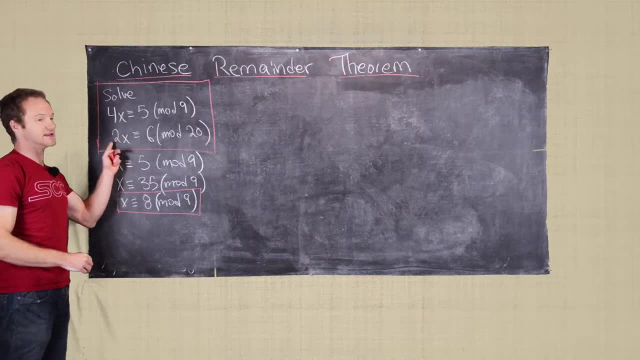 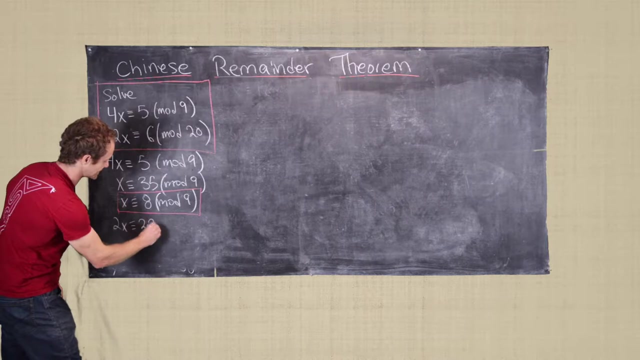 So we notice that 2 is not invertible mod 20, but all three of these numbers are even, so we can take advantage of that. So we'll write this thing as 2x is congruent to 2 times 3 mod 9.. 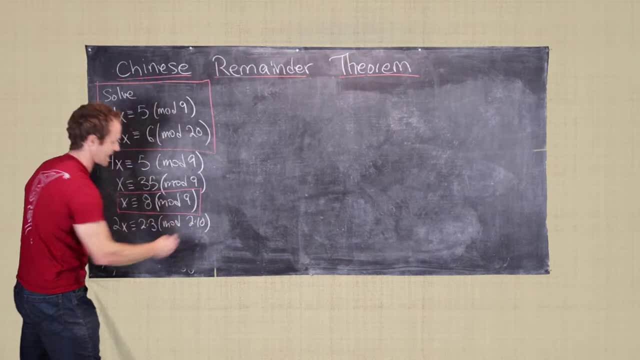 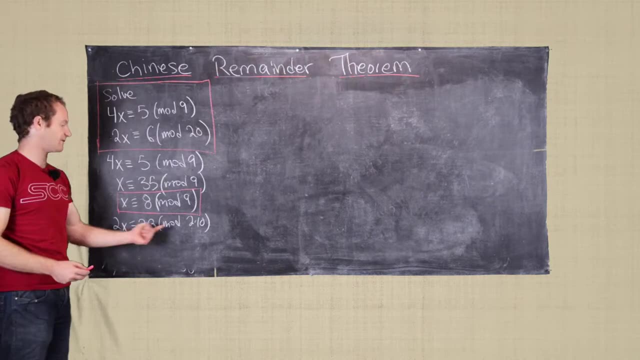 So we'll write this thing as 2x is congruent to 3 mod 2 times 10.. And there was a result that I've proved earlier on the channel that if you have a setup like this, you can cancel the common factor from all three of these parts. 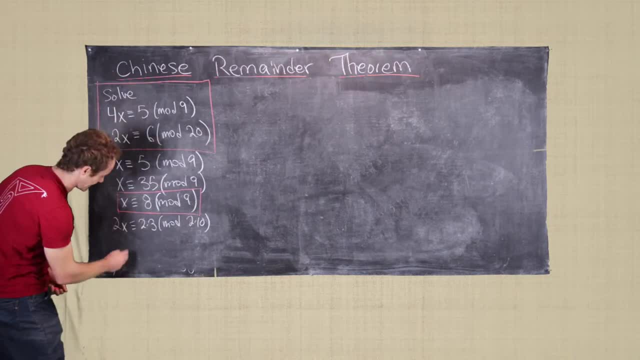 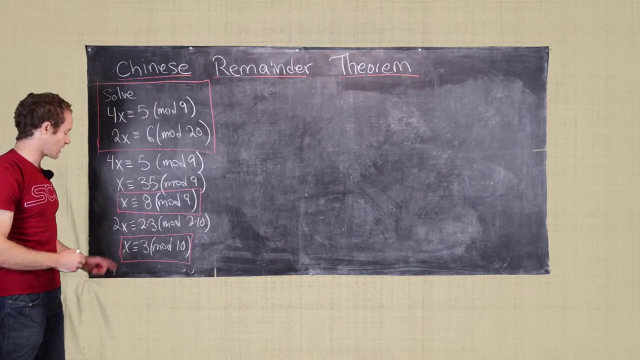 So we can cancel this. 2, and we're left with x is congruent to 3 mod 10.. Good, So now we have a new system of linear congruence. Linear congruence is to solve. We have reduced this to the following. 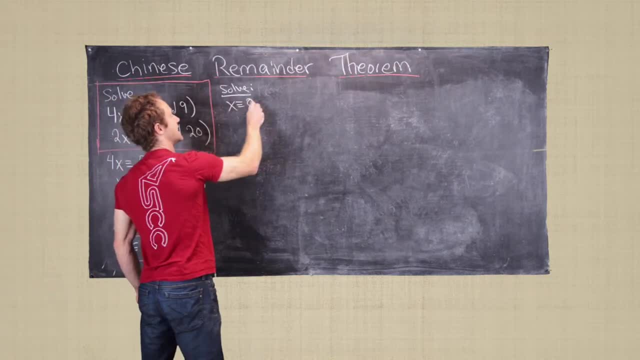 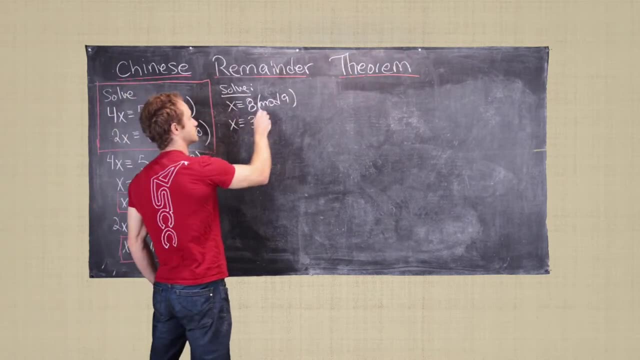 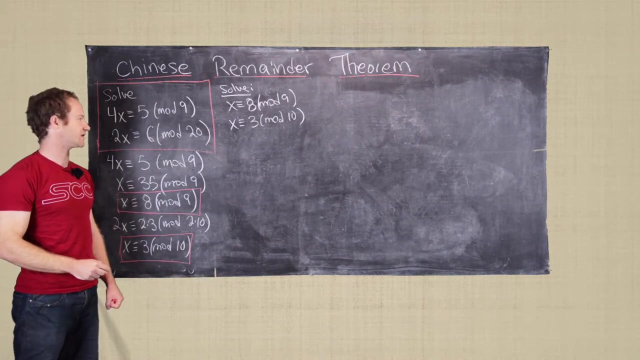 Solve: x is congruent to 8 mod 9, and x is congruent to 3 mod 10.. So that won't be exactly the same as the original linear equivalence because we don't have this mod 20, but we can take care of that at the very end. 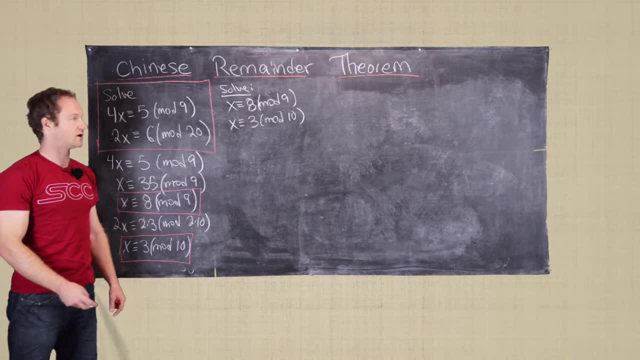 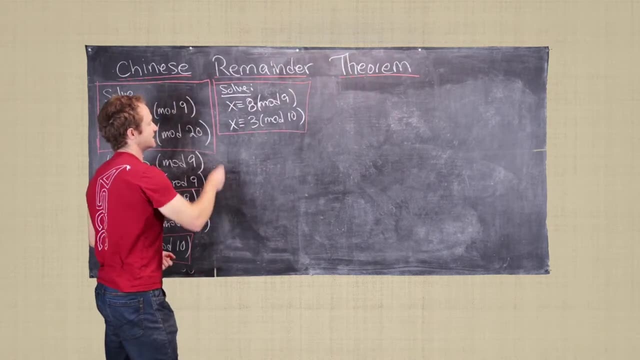 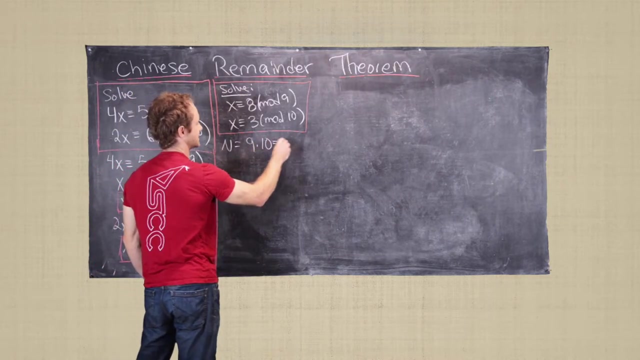 Okay, good, And this thing is set up to solve using the Chinese remainder theorem, So let's do that. So we need to set capital N equal to the product 9 times 10.. So 9 times 10,, so that's 90.. 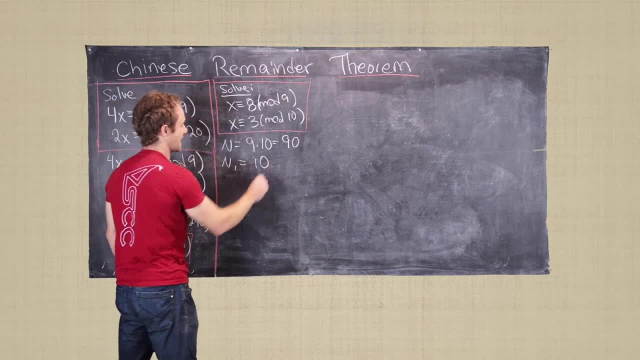 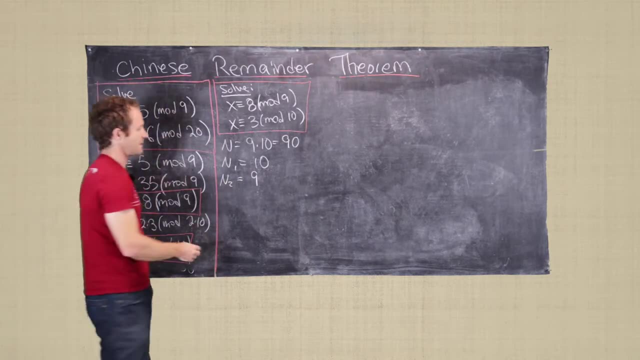 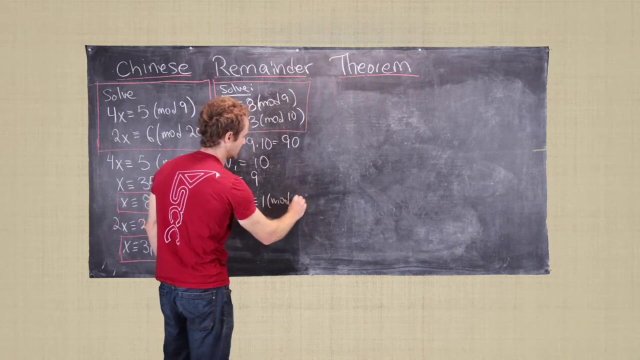 And then capital N1 will be 10.. And then capital N2 will be 9.. Good, so we have that, And then recall that we want to solve this. Nixi is congruent to 1 mod little ni, So these xi's are important to constructing the solution. 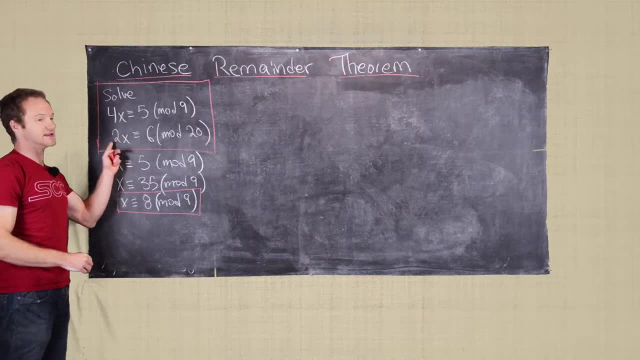 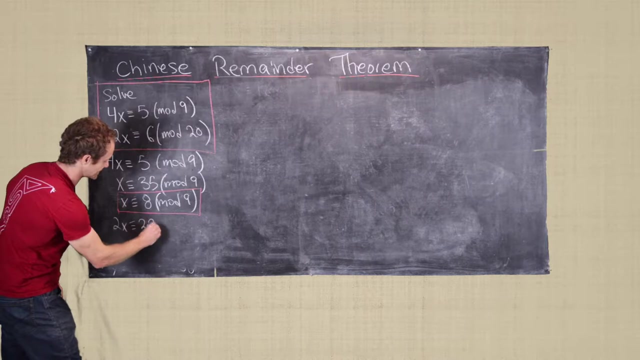 So we notice that 2 is not invertible mod 20, but all three of these numbers are even, so we can take advantage of that. So we'll write this thing as 2x is congruent to 2 times 3 mod 9.. 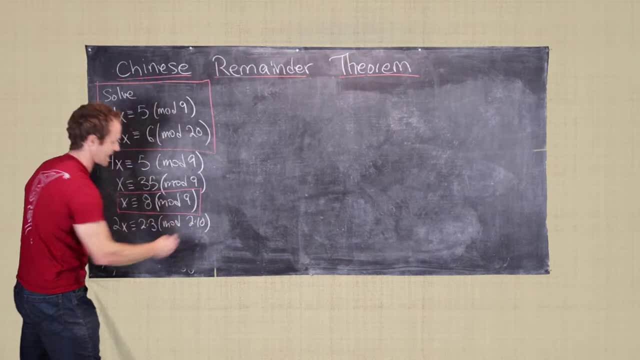 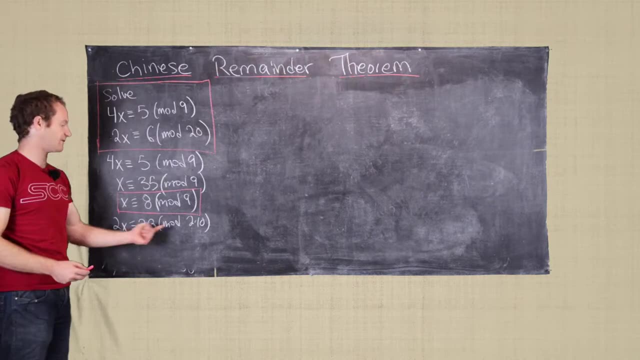 So we'll write this thing as 2x is congruent to 3 mod 2 times 10.. And there was a result that I've proved earlier on the channel that if you have a setup like this, you can cancel the common factor from all three of these parts. 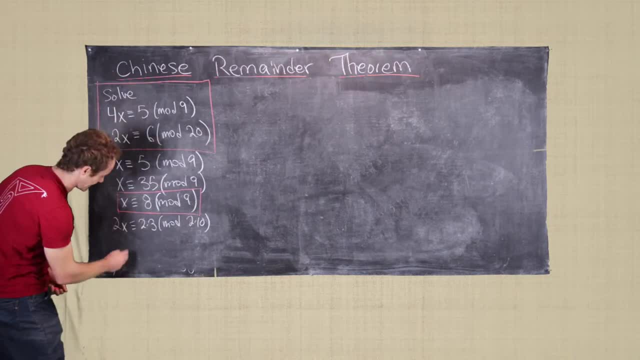 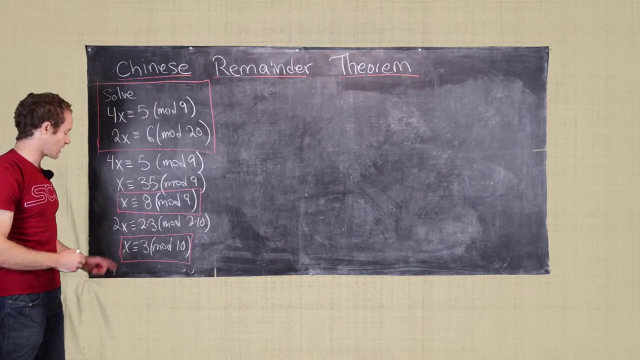 So we can cancel this. 2, and we're left with x is congruent to 3 mod 10.. Good, So now we have a new system of linear congruence. Linear congruence is to solve. We have reduced this to the following. 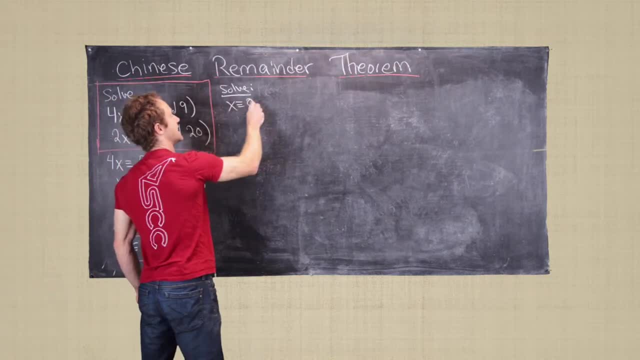 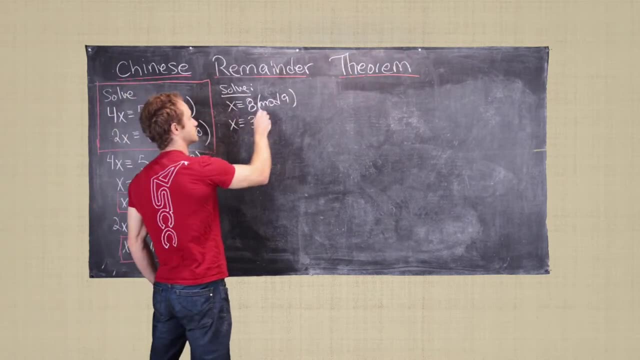 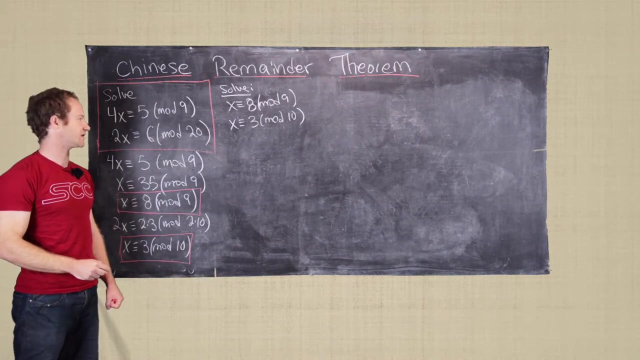 Solve: x is congruent to 8 mod 9, and x is congruent to 3 mod 10.. So that won't be exactly the same as the original linear equivalence because we don't have this mod 20, but we can take care of that at the very end. 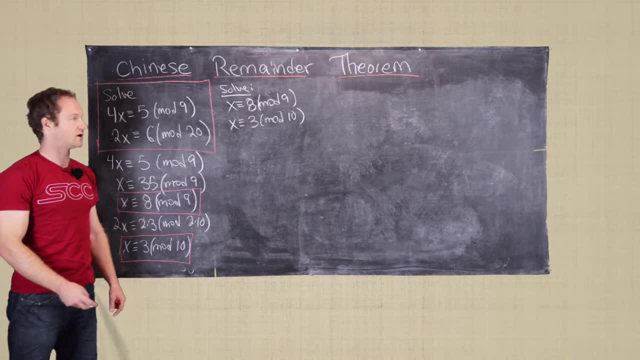 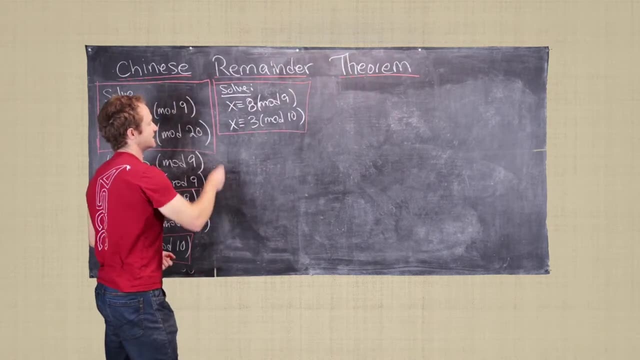 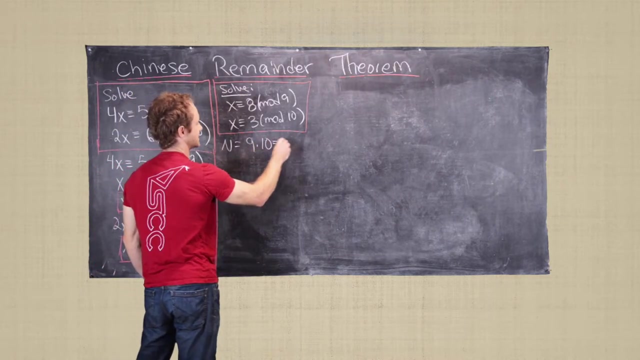 Okay, good, And this thing is set up to solve using the Chinese remainder theorem, So let's do that. So we need to set capital N equal to the product 9 times 10.. So 9 times 10,, so that's 90.. 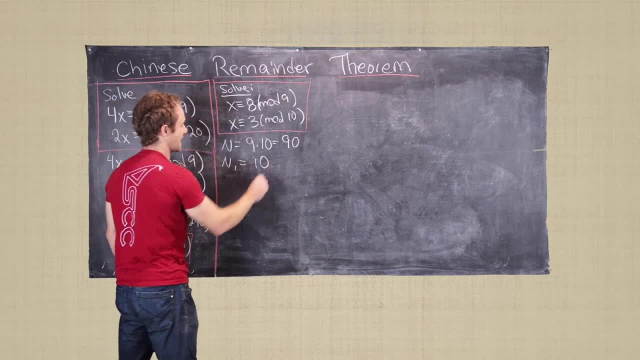 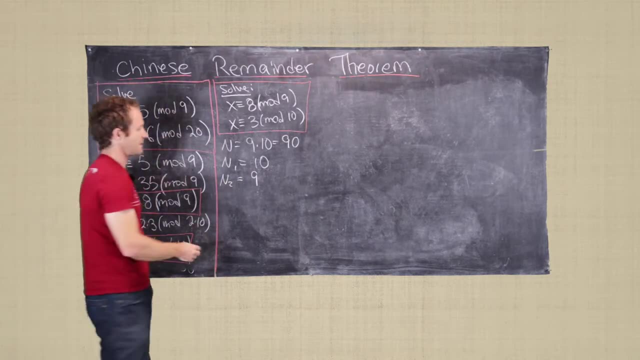 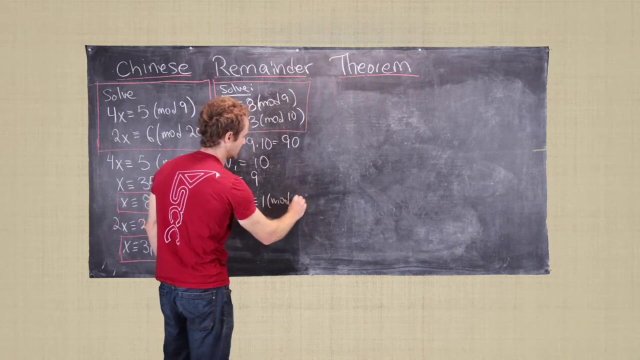 And then capital N1 will be 10.. And then capital N2 will be 9.. Good, so we have that, And then recall that we want to solve this. Nixi is congruent to 1 mod little ni, So these xi's are important to constructing the solution. 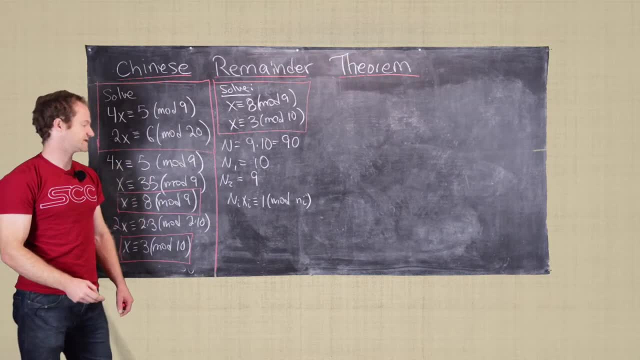 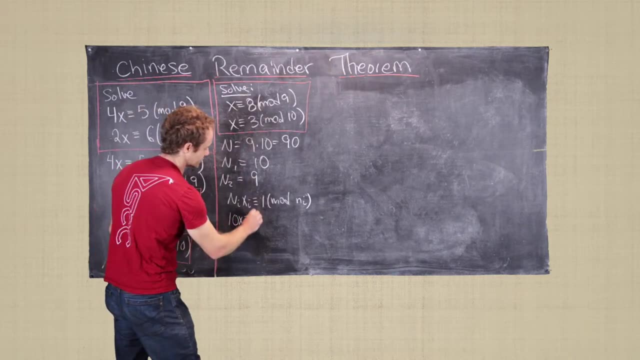 So little n1 is 9 and little n2 is 10.. So that means we want to solve: 10 is congruent, So 10x1 needs to be congruent to 1 mod 9.. But notice, 10 is congruent to 1 mod 9.. 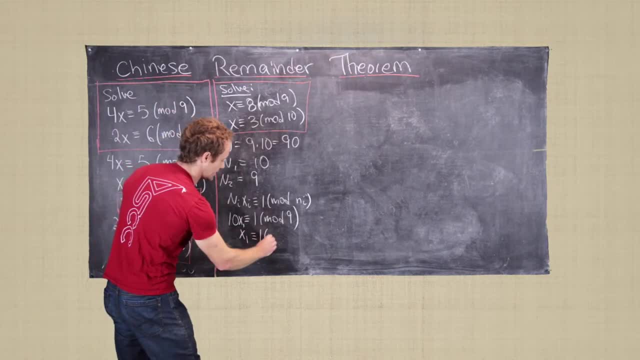 So that means we get x1 is congruent to 1 mod 9.. So that means we get x1 is congruent to 1 mod 9.. So that means we get x1 is congruent to 1 mod 9.. 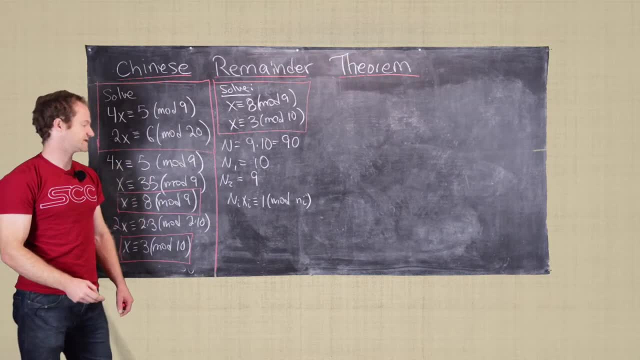 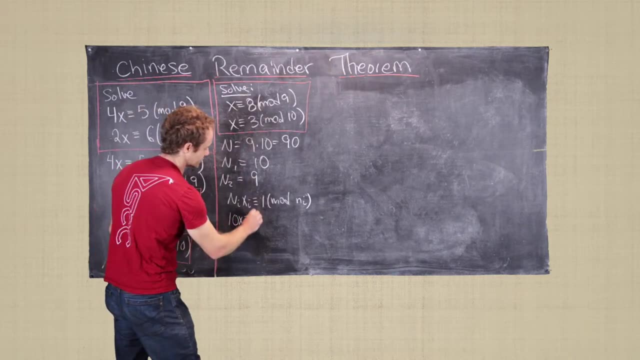 So little n1 is 9 and little n2 is 10.. So that means we want to solve: 10 is congruent, So 10x1 needs to be congruent to 1 mod 9.. But notice, 10 is congruent to 1 mod 9.. 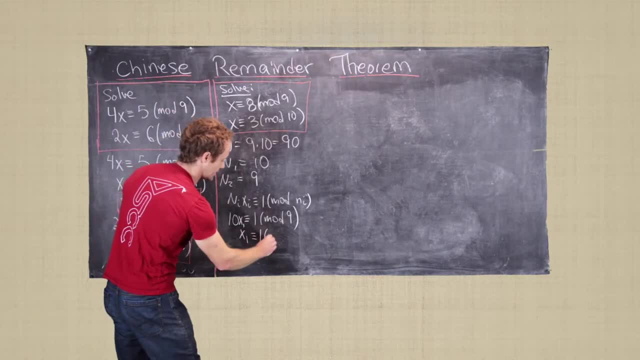 So that means we get x1 is congruent to 1 mod 9.. So that means we get x1 is congruent to 1 mod 9.. So that means we get x1 is congruent to 1 mod 9.. 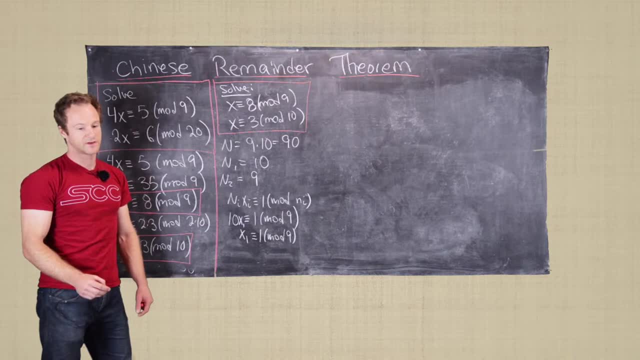 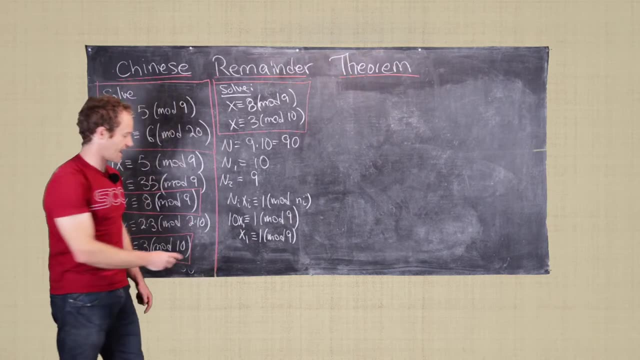 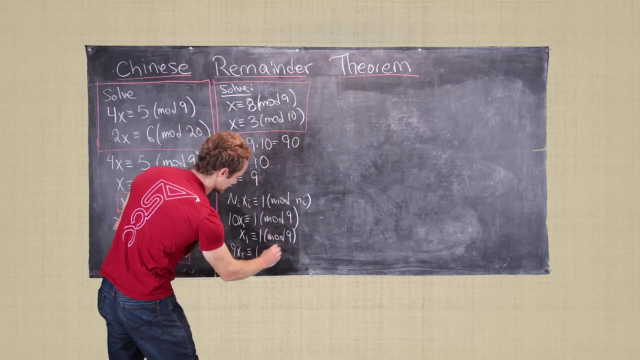 Okay, so that's good. So the next thing we need to do is the following: So now we can write this as 9x2 is congruent to 1 mod 10.. And we notice that 9 times 9 is 81,, which is 1 mod 10.. 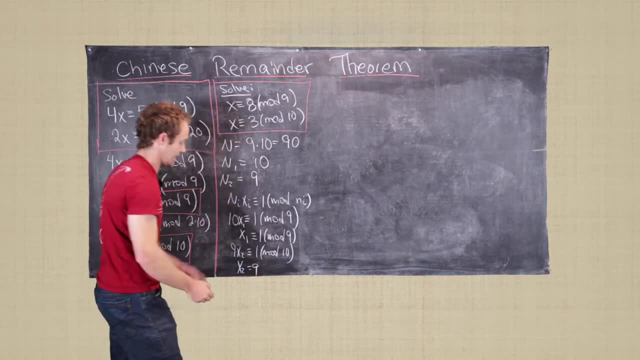 So that means x2 is congruent to 1 mod 10.. And we notice that 9 times 9 is 89,, which is 1 mod 10. So we have: x1 is 1 and x2 is 9.. 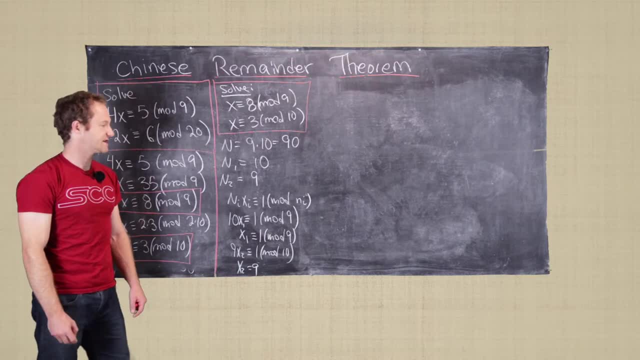 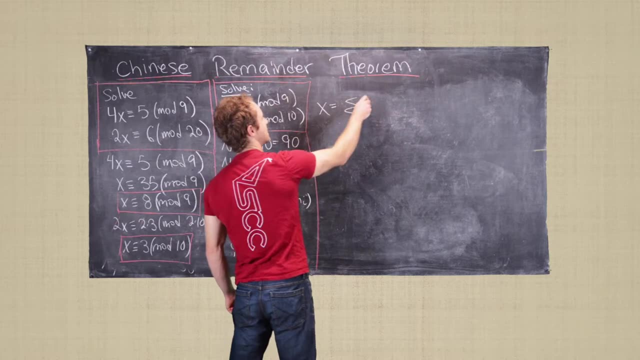 So let's go back to this first problem. We have: x1 is 1 and x2 is 9.. Okay, fantastic. Now we can go on to the next step of constructing our solution. So we wanna set x equal to the sum of the xi, the ni and the bi. 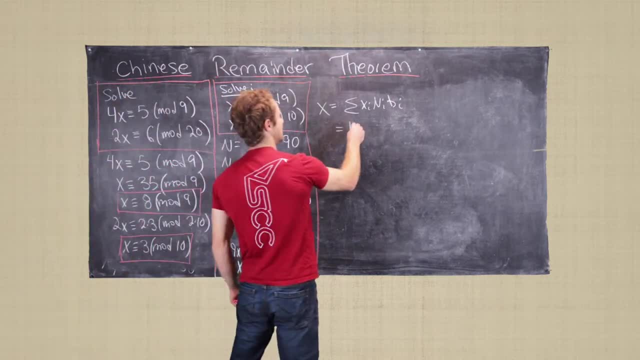 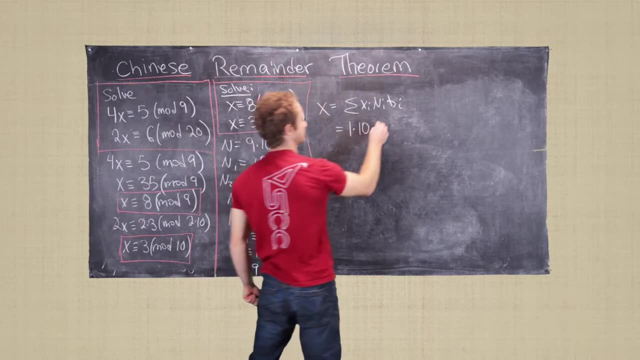 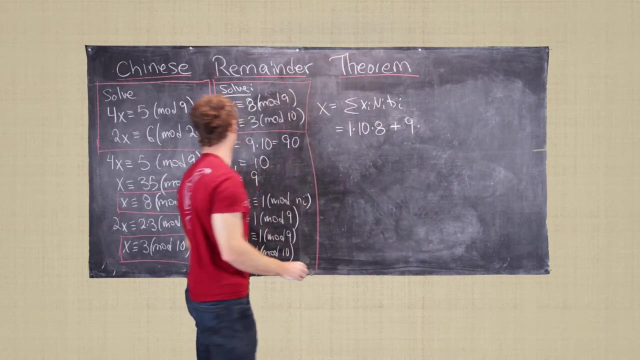 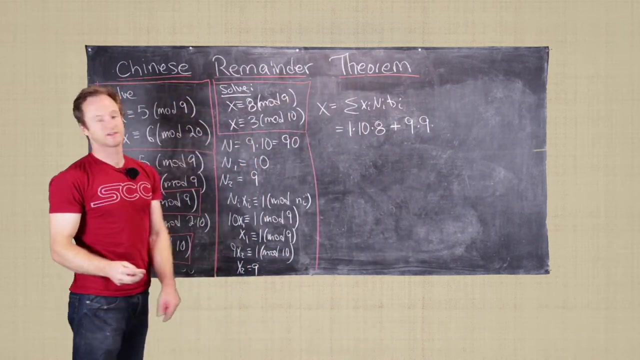 So that's gonna be x1,, 1x, n1, which is 10x. mi doesn't matter, because two controls in turns: OK, which is 8,, plus x2, which is 9, times n2,, which is 9, times b2, which is 3.. 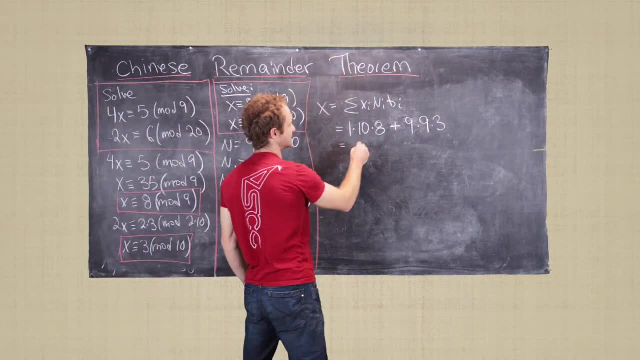 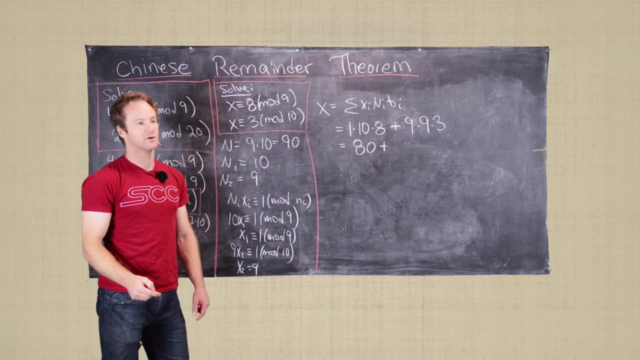 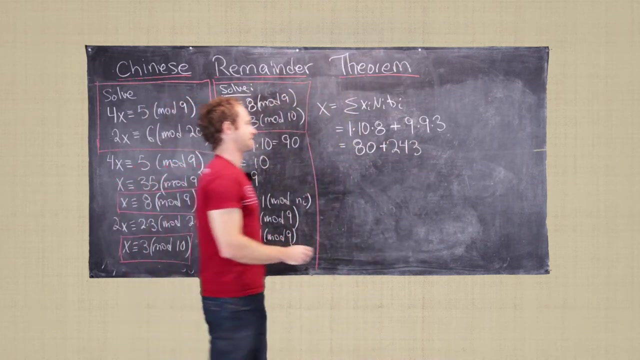 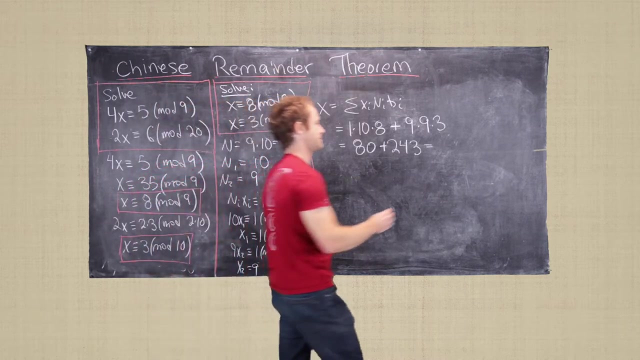 Good. So now notice that is going to give us 80 plus 81 times 3.. So 81 times 3 is 243.. Good, So we have 243.. So that tells us that x is equal to 323.. Good. 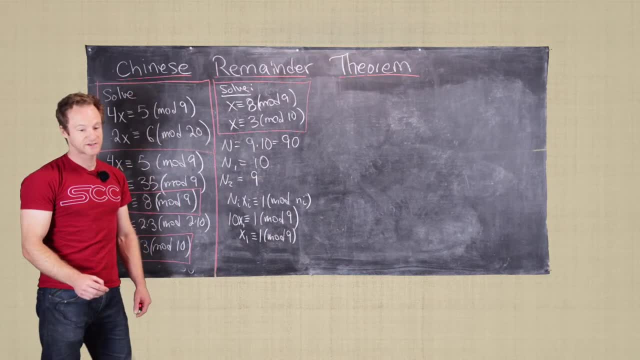 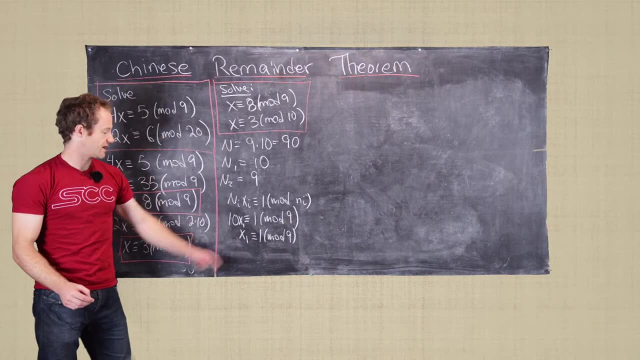 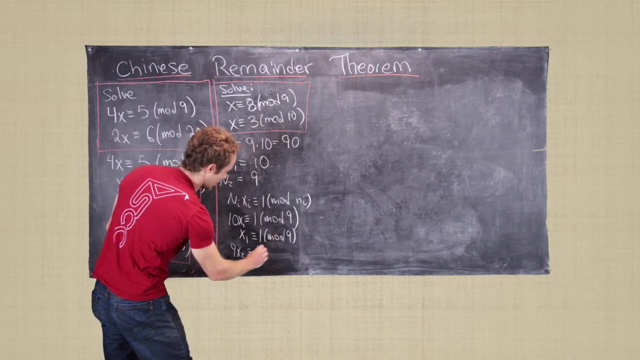 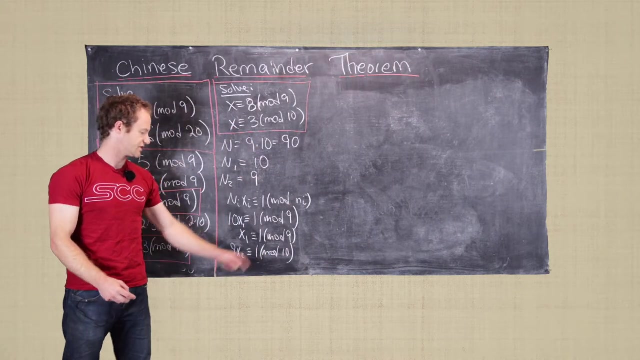 Okay, so that's good. So the next thing we need to do is the following: So now we can write this as 9x2 is congruent to 1 mod 10.. And we notice that 9 times 9 is 81,, which is 1 mod 10.. 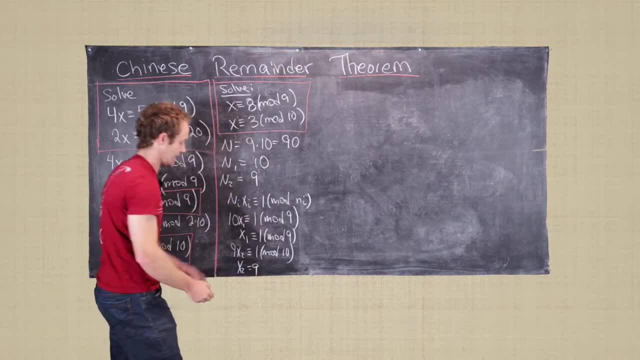 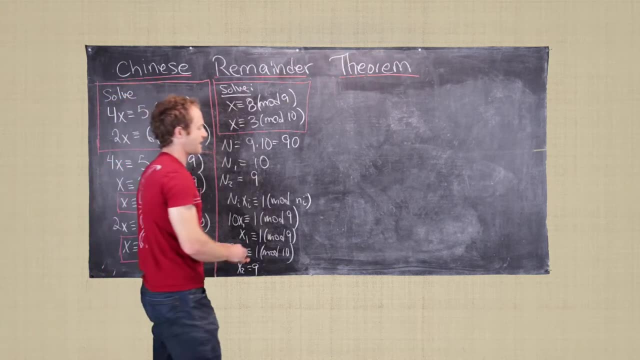 So that means x2 is congruent to 1 mod 10. x2 we can take to be 9.. So we have: x1 is 1 and x2 is 9.. Okay, fantastic, Now we can go on to the 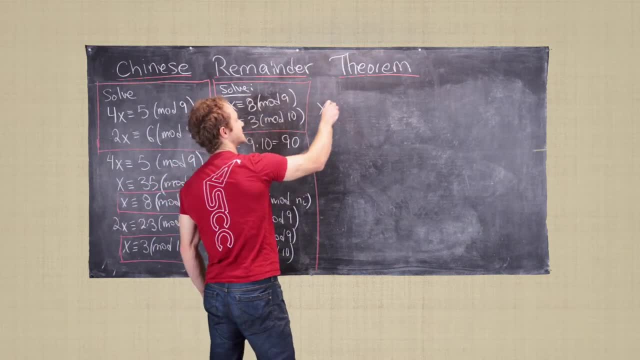 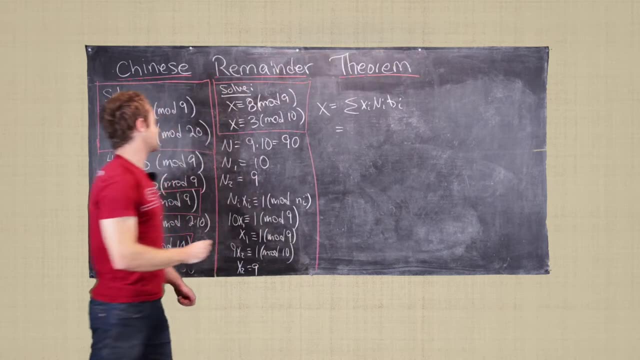 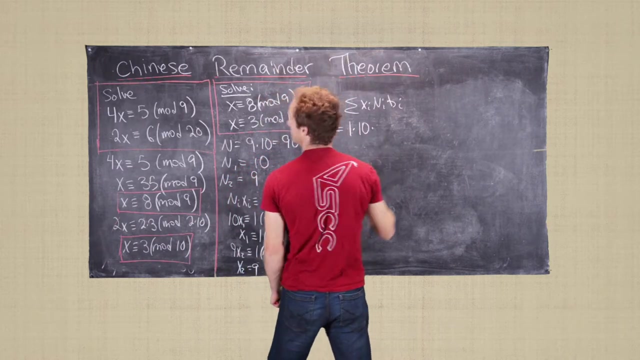 next step of constructing our solution. So we want to set x equal to the sum of the xi, the ni and the bi. So that's going to be x1, 1 times n1, which is 10 times b1, which is 8. 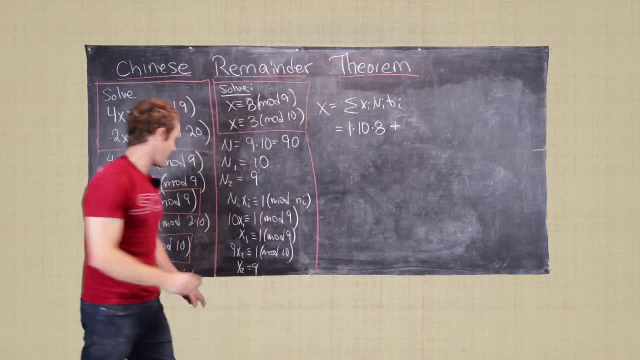 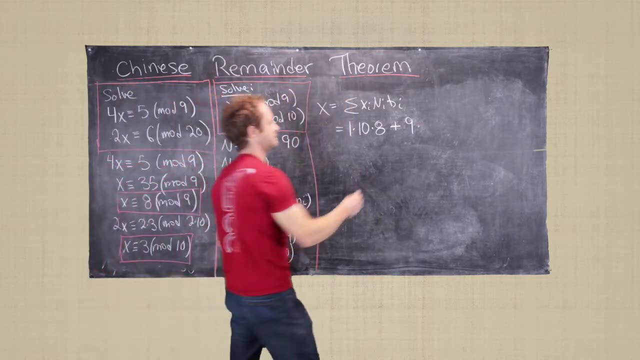 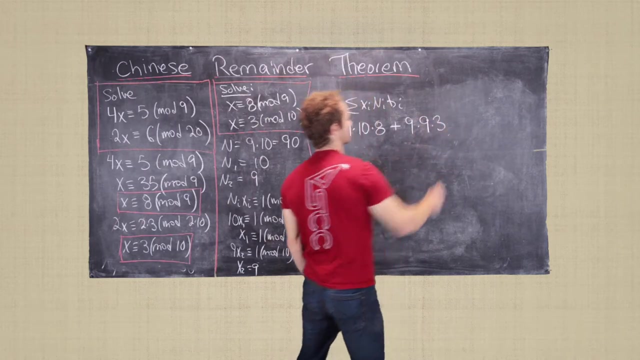 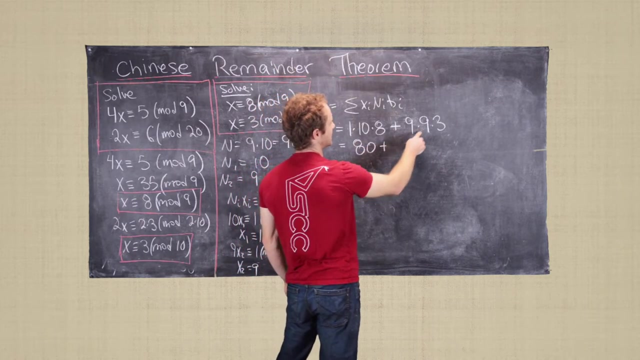 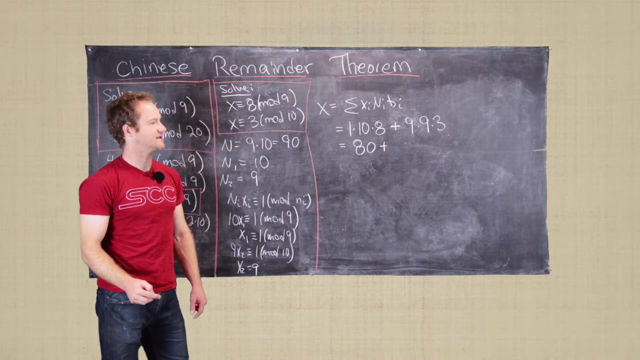 plus x2, which is 9 times n2, which is 9 times b2, which is 3.. Good, So now notice that is going to give us 80 plus 81 times 3.. So 81 times 3 is 243.. Good, 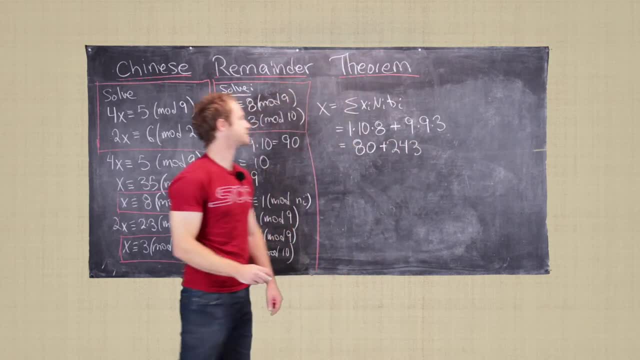 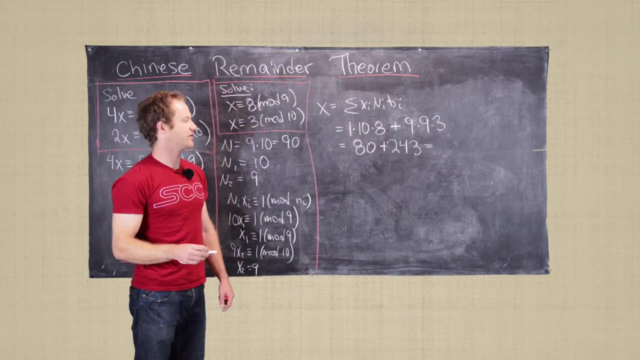 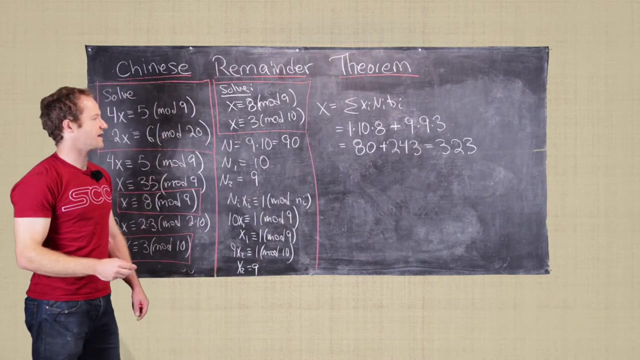 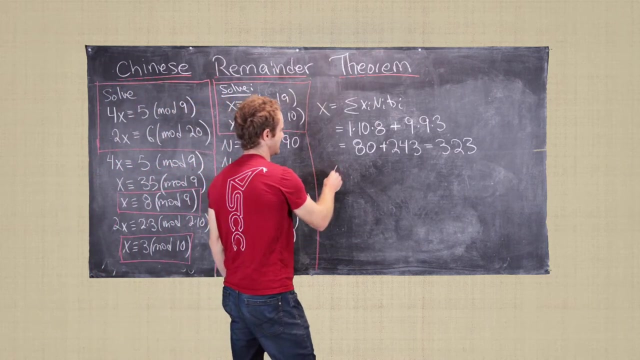 So we have 243.. So that tells us that x is equal to 323.. Good, But now we know by the Chinese remainder theorem that this should be unique modulo 90. So that means x is congruent to. so we need to reduce this mod 90. So 270 will be. 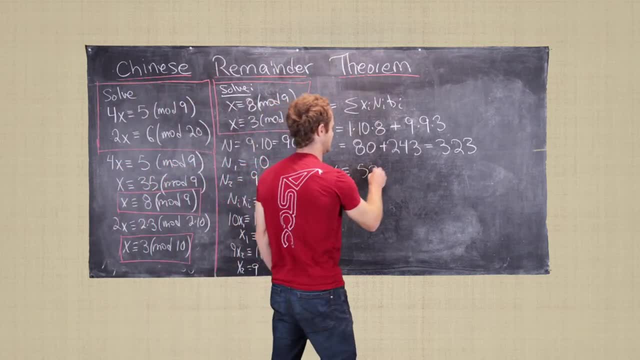 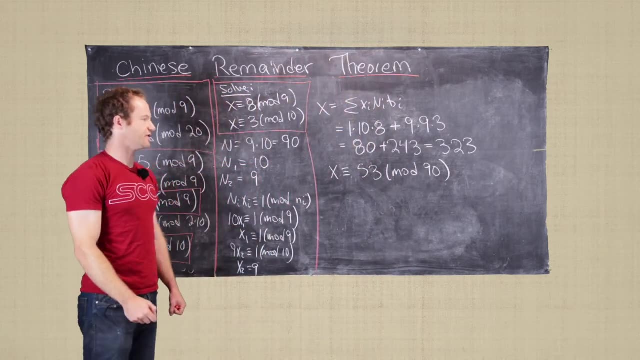 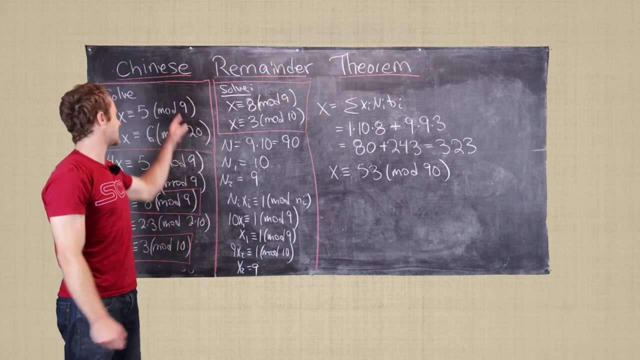 the closest. So that's 53.. 53 mod 90.. Good, So we have a unique solution- mod 90.. But we want to solve this- maybe mod 180, because that's the product of these two, And so we can do that, And that means we have two solutions.